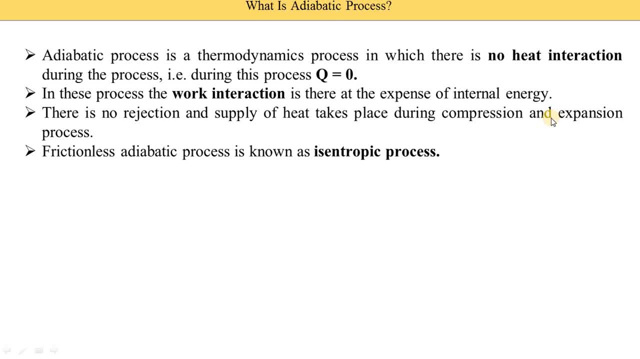 the component are moved without friction means pistons are moving without frictions. then it's followed isentropic process. okay, so generally, for the compression process we require the compressor. for the expansion process we require the turbines. okay, so this compressor and the turbine have a lots of moving component is there and in the moving component there is a friction. 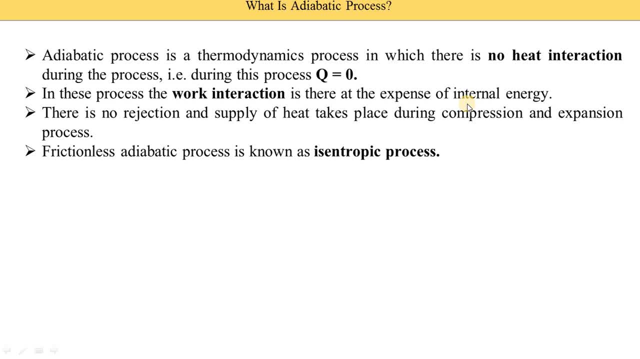 is there? okay, it is not possible to run the compressor and the turbine without frictions. okay, and suppose we can run this compressor and turbine frictionless. then this adiabatic process is called as the isentropic process. now let gas contain in a piston cylinder. 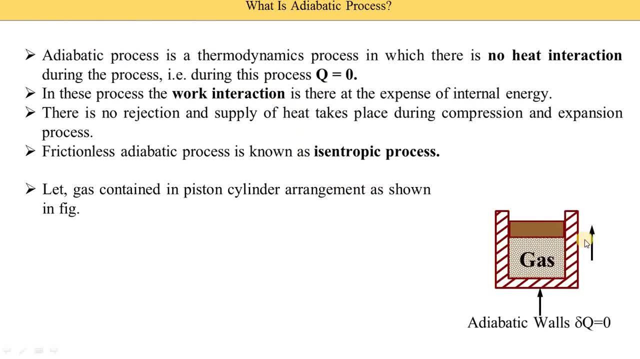 arrangement as shown in this figure. so here now, here you see the figure of cylinder piston arrangement. this is the cylinder, this is the piston, and in between this piston and cylinder gas is filled at. okay, and here we mentioned that is the adiabatic wall. is that adiabatic wall means? 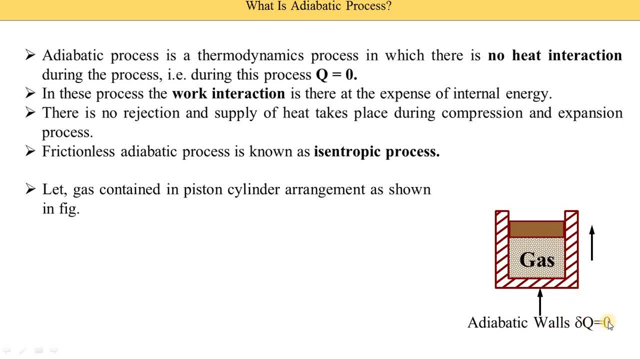 it is. the insulated wall is there, and here we mentioned the del. q is equal to zero, means we are not supplying any heat, and the it is not rejected from the gas to the surroundings. and this is the piston, and these pistons are moving up and down. okay, on the basis of that, the compression 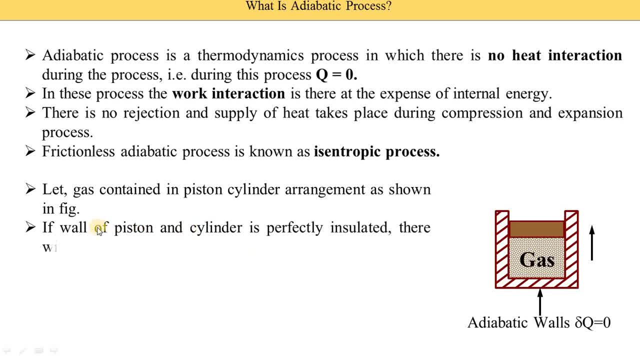 expansion is going on. if wall of piston and cylinder is perfectly insulated, there will be a no heat transfer to or from the systems. okay means avoid these heat interactions. we need to do the insulation of the cylinders okay and when we do this insulation then the heat is not inter. 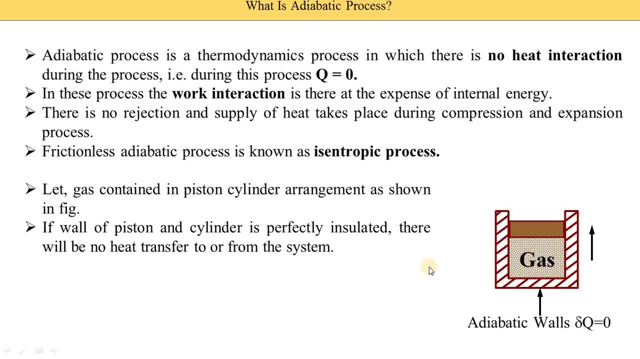 in the system and heat is not go away from the system. it is called as the 2n from the system. gas can be compressed or a expand. an internal energy of the system will be increased or increased. okay, so when we do this compression, when this piston is moving in, 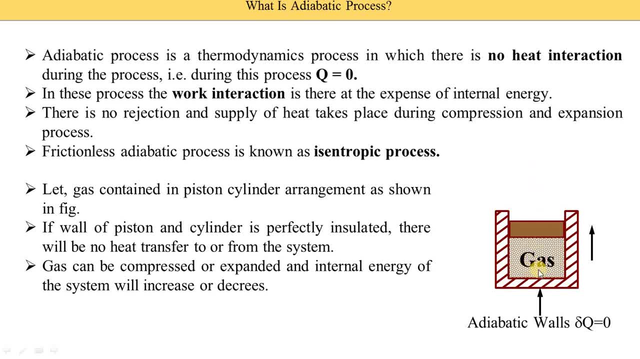 this downward direction, at that time this gas is compressed and volume is reduced. when this piston is moving in this upper direction, at that time the gas volume is increased. it is called as the expansions and on this basis of this compression and expansions, the its internal energy of the